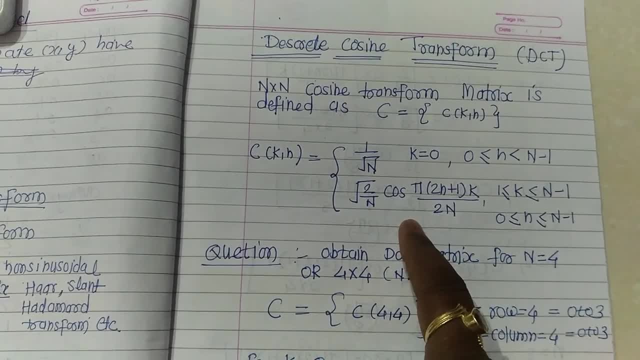 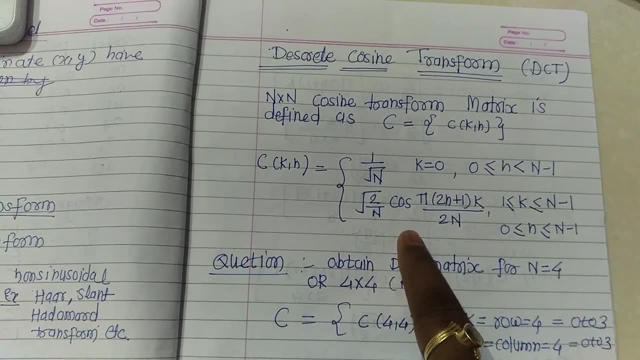 image from one form to another form. We have to modified image. So for that purpose we have to use the transform. Each of the transform is having the different application. The DCT will be used for the image compression. So the question can be asked: obtain the DCT? 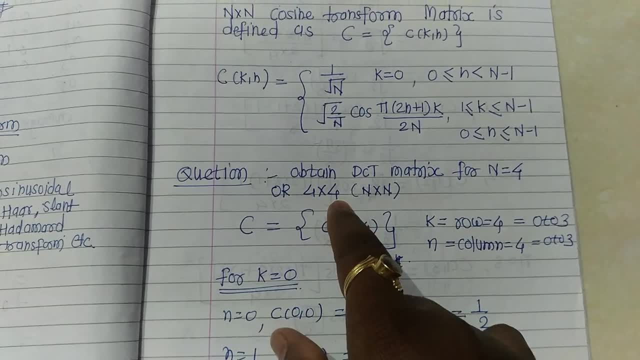 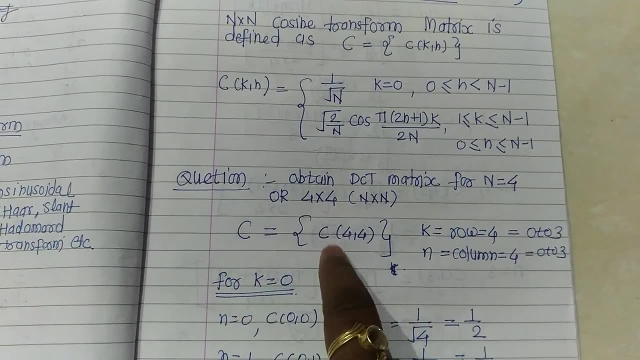 matrix for n equal to 4.. So the answer is 4 by 4 matrix. So we have to generate the DCT matrix for 4 by 4.. Again, here, first of all, we write: c is equal to c, k, comma, n, where k and n, that is the rows. 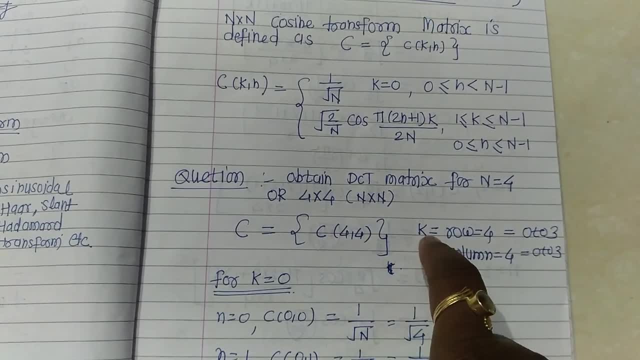 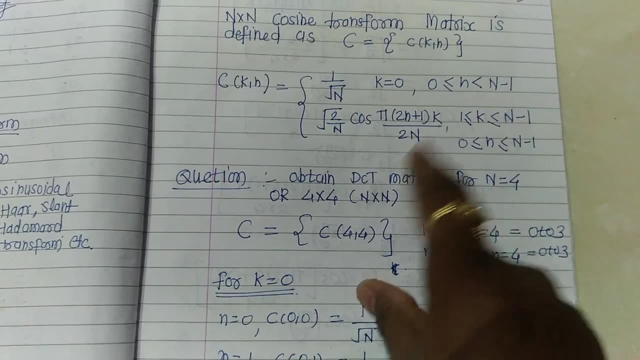 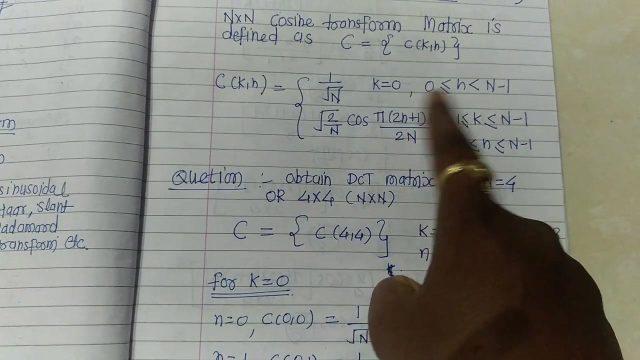 and column are 4, 4.. So again we have to determine the range of k and n. The range of k is from 0 to n minus 1.. So n is 4.. So it is 0 to 3.. It is the range of k and the range of n is. 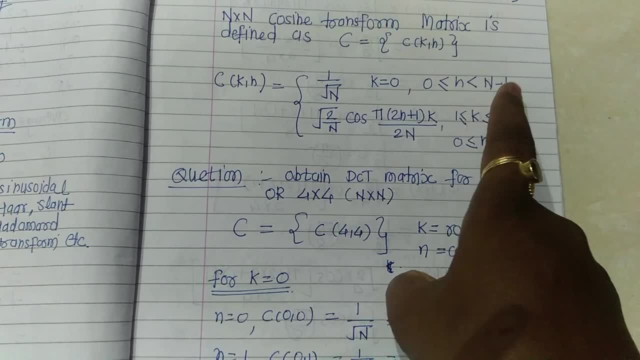 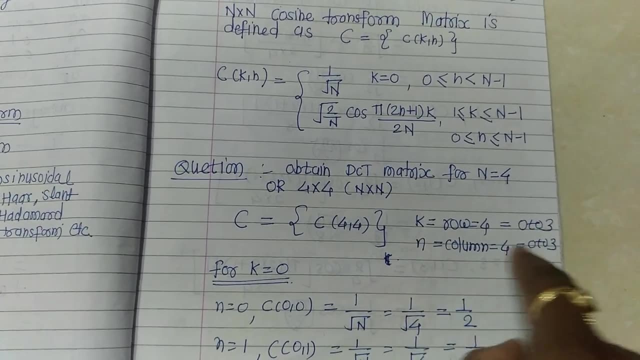 0 to n minus 1. for both, the equation That is 0 to 4 minus 1. That is 0 to 3. So that is the range of k and n. That is 0 to 3.. Again, k and n is 0 to 3. So we have to determine. 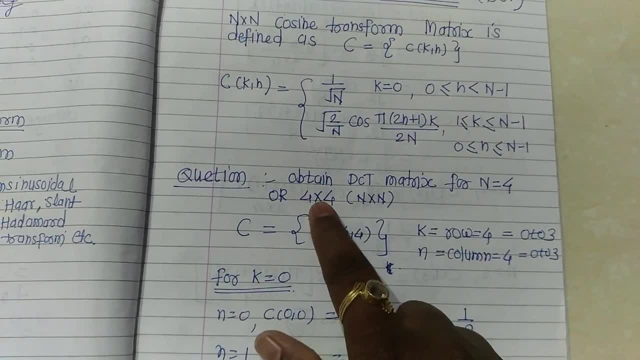 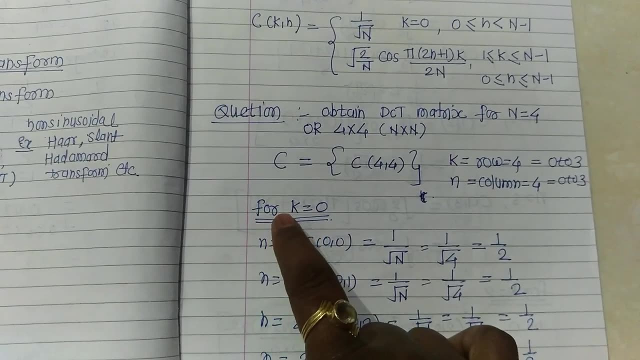 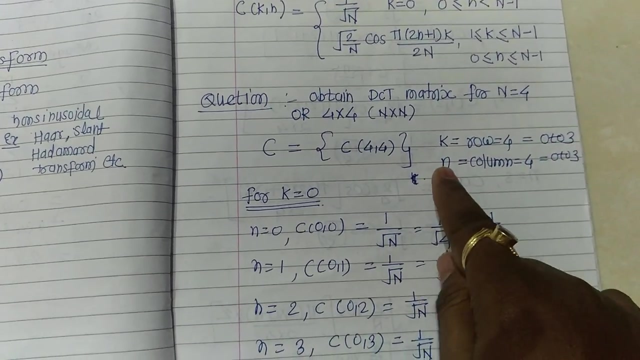 first the range of k by using the value of n, by using this above equation, Now we have to determine the DCT matrix elements. For that we have to vary the k from 0 to 3 and in under this we have to vary the k from 0 to 3.. So we have to vary the k from 0 to 3.. 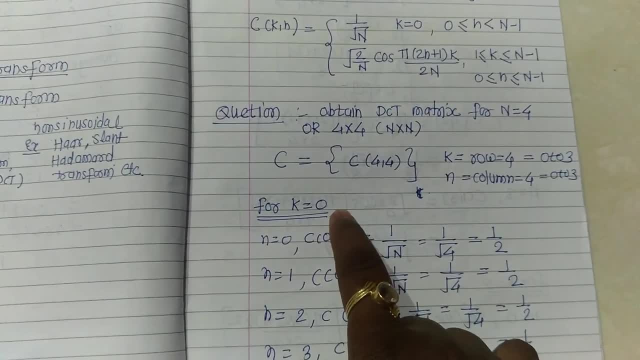 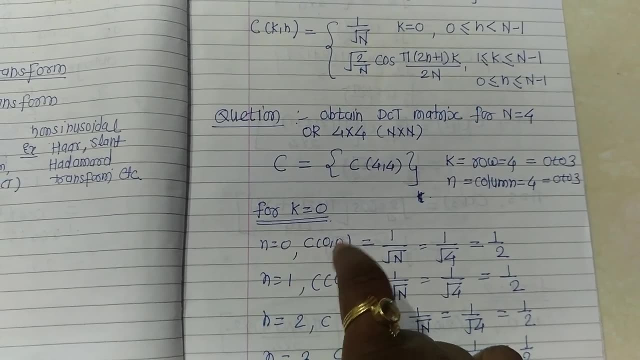 So first of all we have to take: k is equal to 0. So k is equal to 0. For that first we consider n is equal to 0. So c, k, comma, n, that is, both are 0, 0. So rows and column, both. 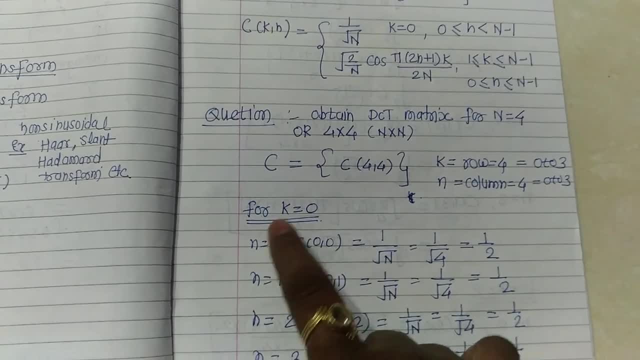 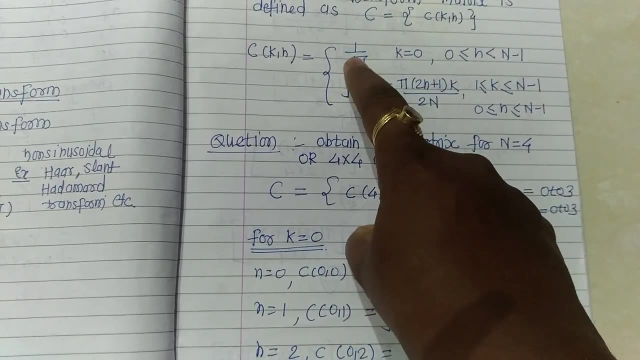 are 0, 0. The first element is this, and here the k is 0. Then out of these two equations we have to select the 1 upon root n as k is 0. Then we have to take this value and if 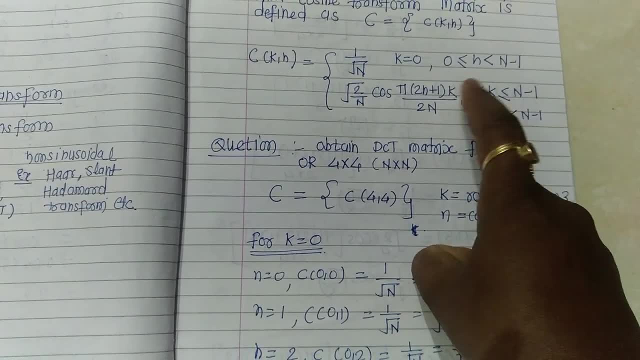 k is between 1 to n minus 1, that is 1 to 4 minus 1.. So we have to take this value and that is 1 to 3. we can take this equation, But in this case the k is 0. So we have to. 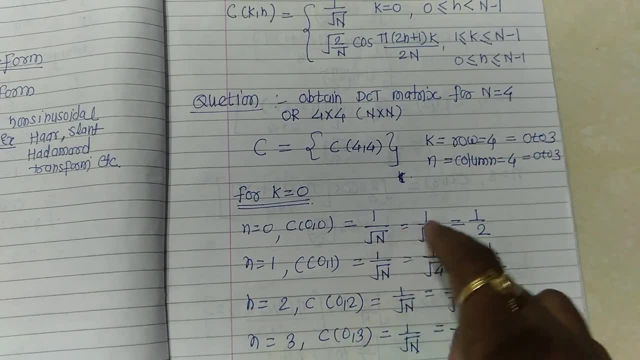 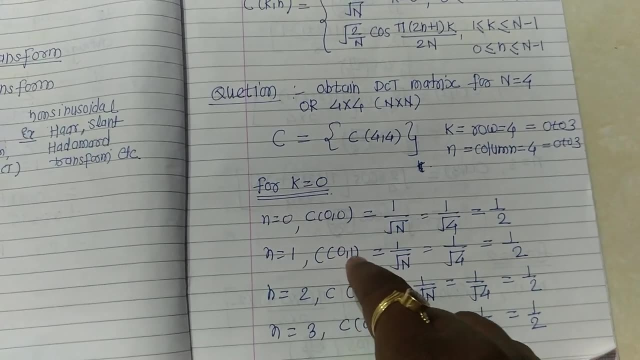 take this equation: 1 upon root n, So 1 upon root n, the n is 4, 1 upon root 4, that is half. Similarly, n equal to 1.. So c k comma n, that is 0 comma 1.. Again, here the k is 0.. 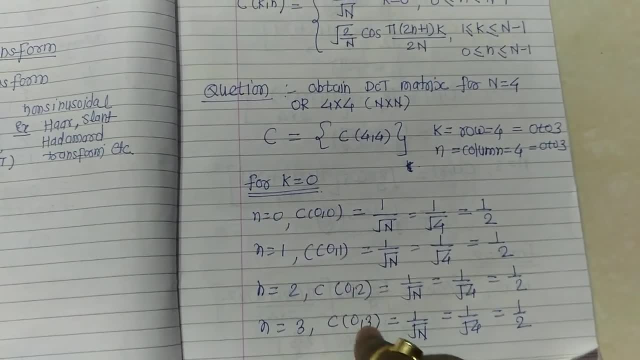 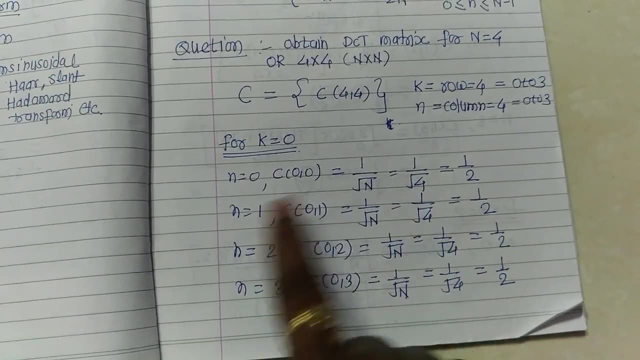 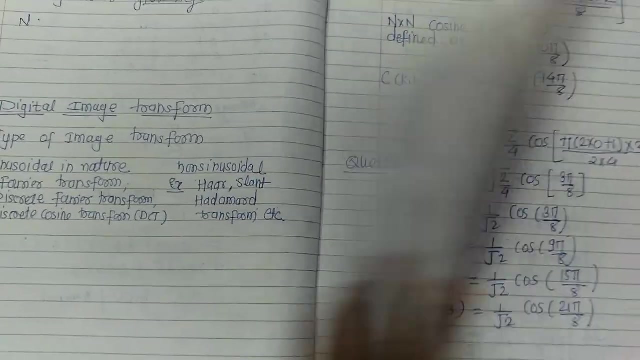 Each of the case here, all for n values, the k is 0. So we have to take the first equation, 1 upon root n. So in this way we determine the first row elements, for k is equal to 1, 0.. After that we have to k: the k equal to 1.. So now here we take the k equal to 1. See. 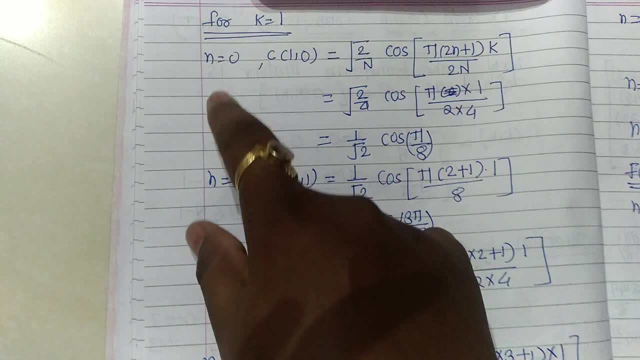 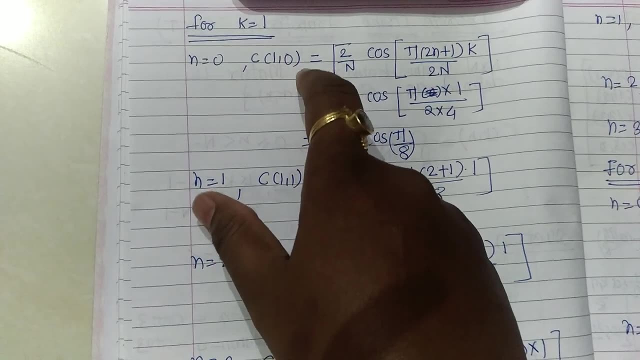 here k equal to 1.. Again, here n is 0 in between. in under this we have to varies the n from 0 to 3. So k equal to 1. So c k comma n, that is, 1 comma 0. So for that case now we have: 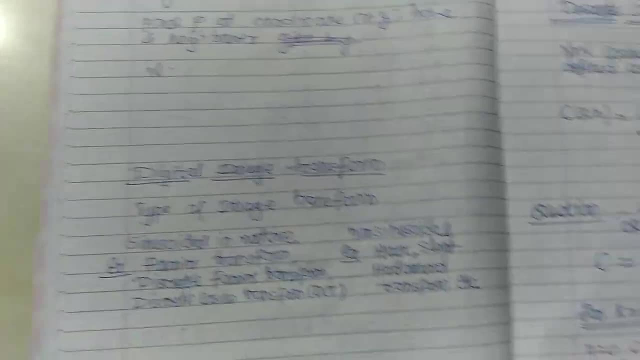 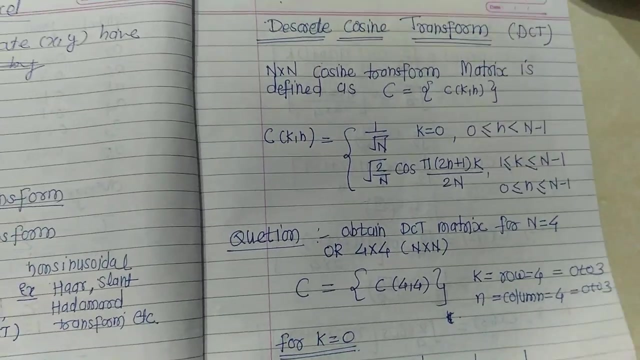 to take the second equation, as k is a 1.. When k is a 1. Then we have to take this equation. when the k varies from 1 to 3. We have to take the second equation. So now we have to take the second equation: when k is equal to 1,, 2 and 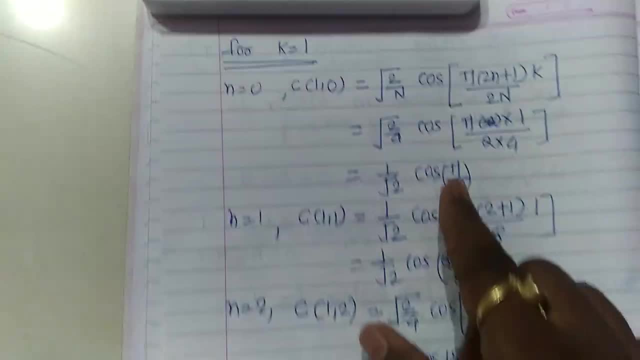 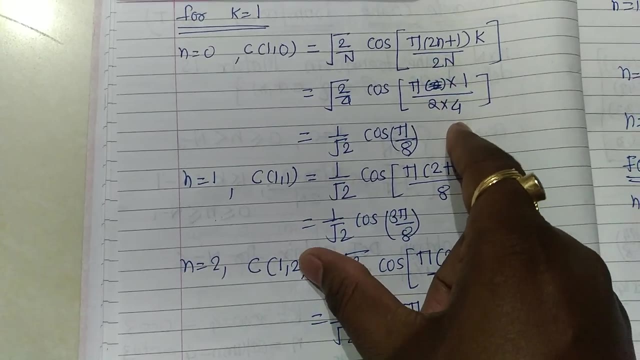 3.. So we have to write this equation that root 2 by n cos pi 2n plus 1k divided by 2n. So here capital n is 4. Put the value and n is 0. Put here the value, We get 2 into. 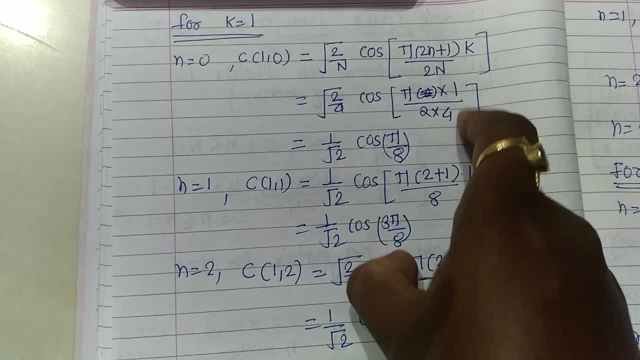 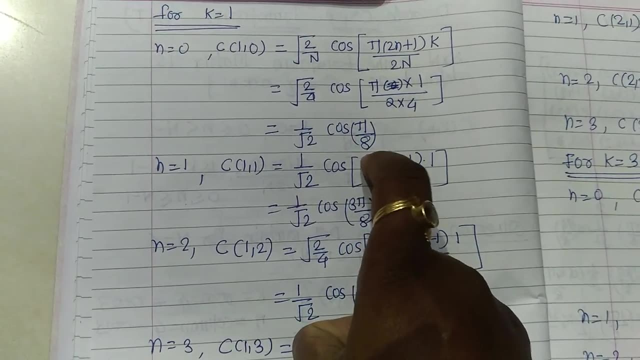 0, that is 0, plus 1, that is pi, and k is 1.. So we are getting 1 upon root. 2 cos pi by 8.. Here the pi is we consider as 180.. 180 by 8.. We have to convert this radian and we have to calculate the cost of this pi by 8.. 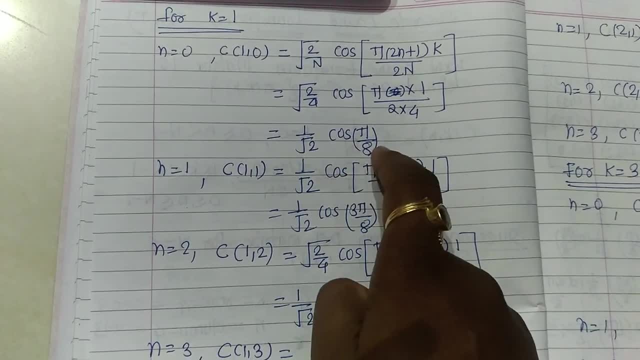 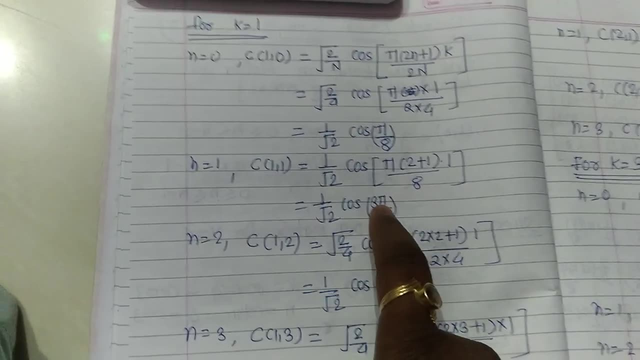 And we can multiply with 1 upon root 2 or we can keep it as it is. Similarly, we have to take the n equal to 1, for that we calculate again the equation. Again. we have to take the same second equation where the k equal to 1, that is root 2, by n, cos, pi, 2n plus 1k. 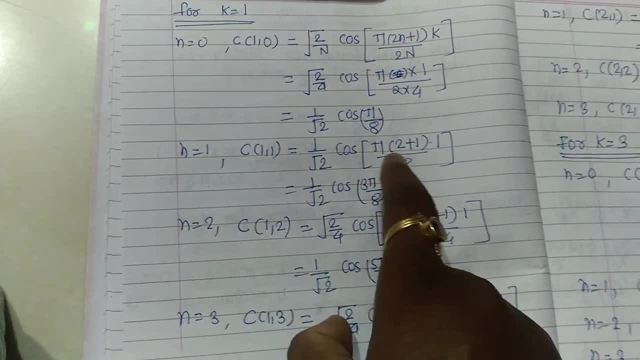 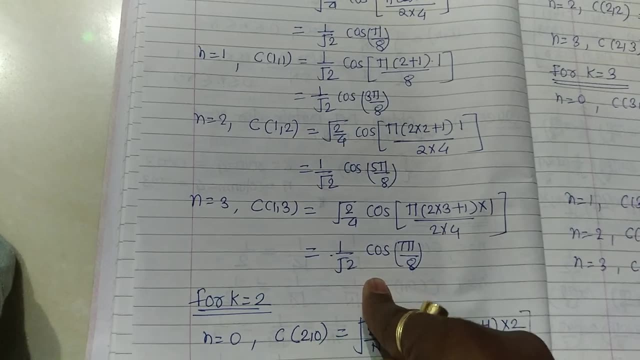 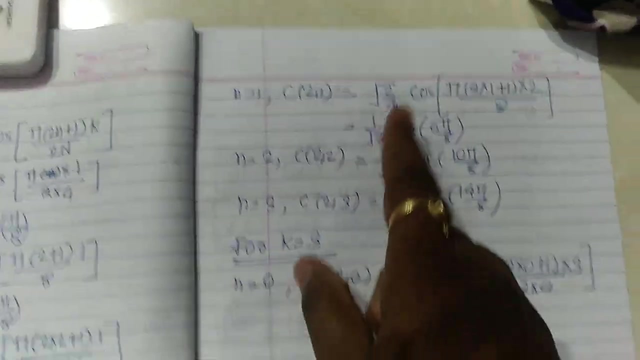 divided by now. here the n is varies where n is 1, so we have to put n equal to 1. so in this way we have to calculate all the values, that is, the value of the second row of DCT matrix. similarly, for k equal to 2, we have to again calculates all the values and after calculating all the values up. 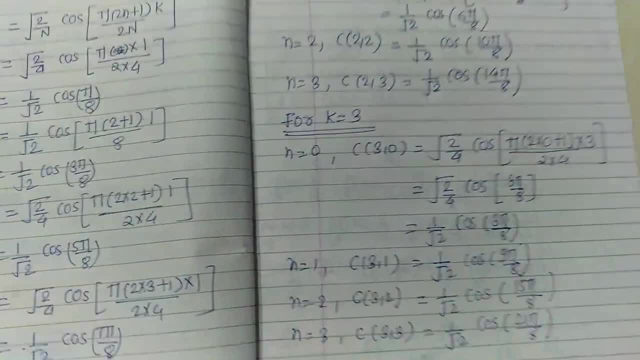 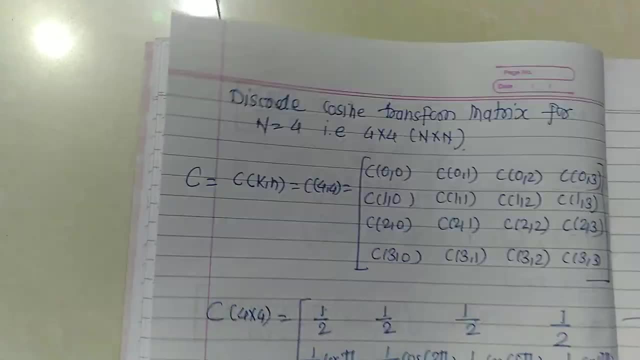 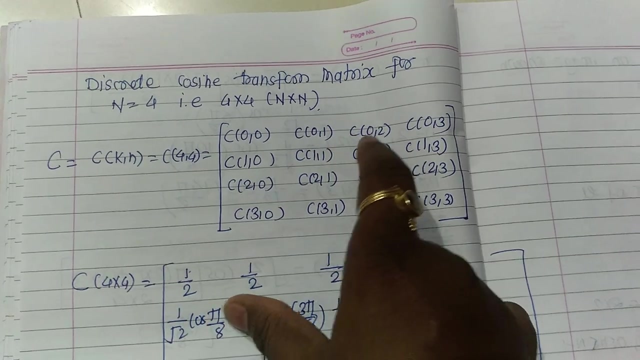 to the k equal to 3, we have to find the DCT matrix and the DCT matrix can be find out. so for 4 by 4 as ckn, that is a 4 by 4, k and n is 4 by 4. so we can write c00, c01, c02, c03, these 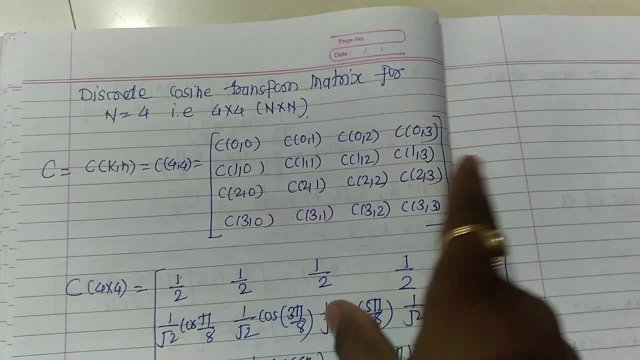 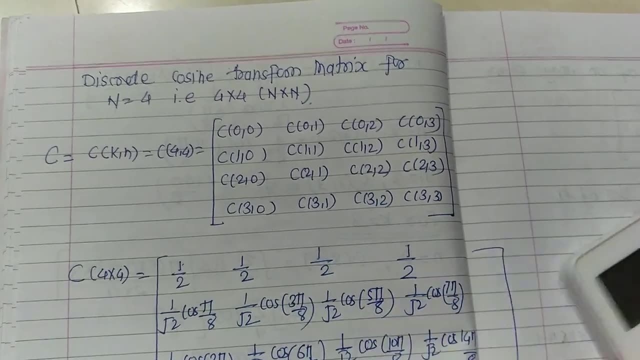 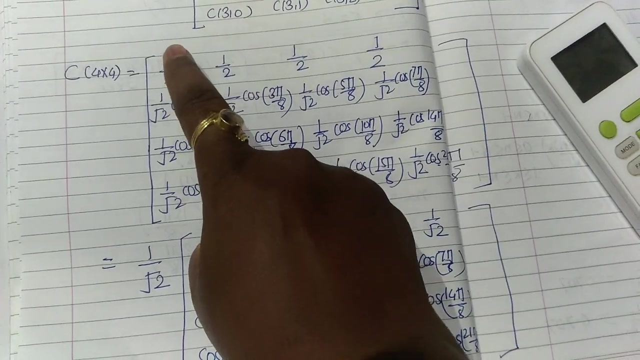 are the first elements of the row, is the second elements of the row, third elements of the row and fourth elements of. we have to find out all this value previously. we have to put this value in this matrix. so finally we get the DCT matrix of the size 4 by so 4. so 1 by 2 can be written as: 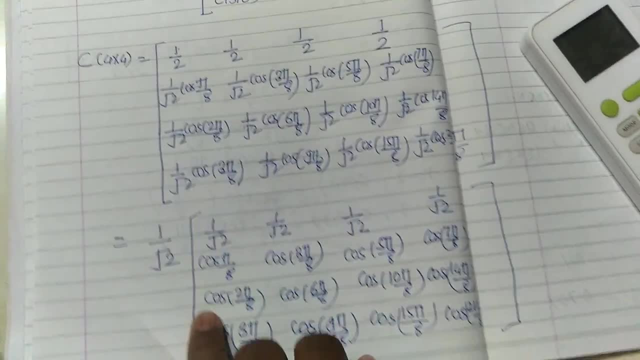 1 of 1,, 5 of 1,, 6 of 1,, 6 of 1, etc. 1 root 2 into root 2. So we can take 1 upon root 2 outside, and after that we get the density. 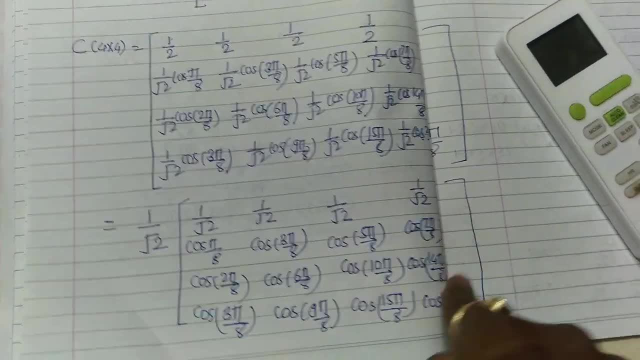 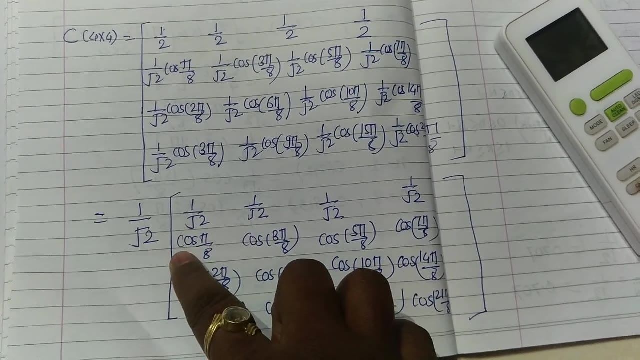 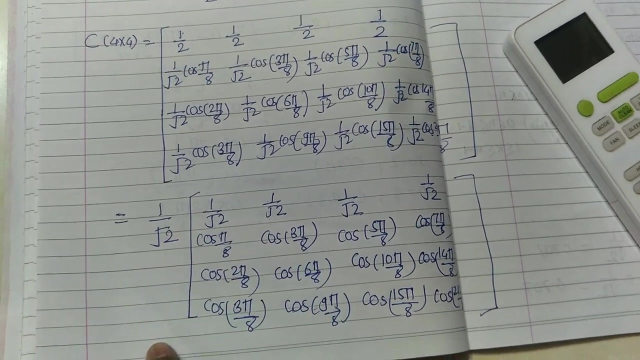 matrix of the size 4 by 4.. So we can also simplify this by converting this pi by 8, that is, 180 by 8, into the degree and calculating the cost of this value. Similarly we can do for the another cost and we can simplify this value or we can keep as it is. So thank, 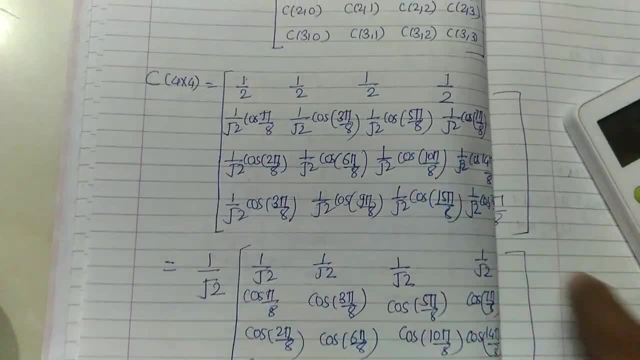 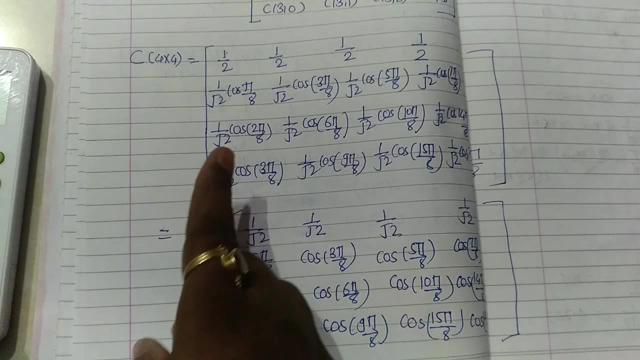 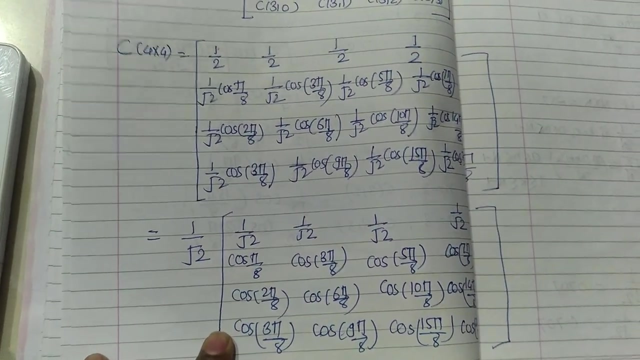 you for watching my video and next video will be the numerical on the DCT: how to solve the numerical on the DCT. This is the basic generation of the DCT matrix of 4 by 4.. We can generate also the 2 by 2, depending on our numerical. how to apply this DCT matrix. 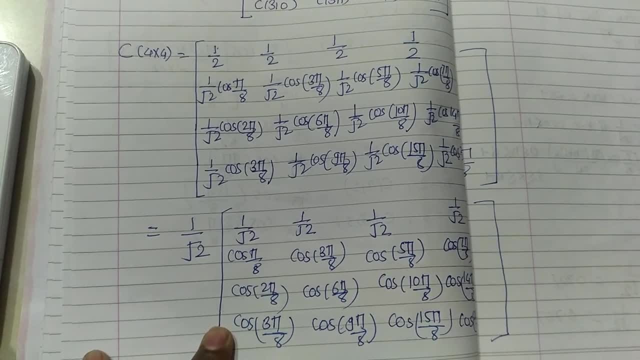 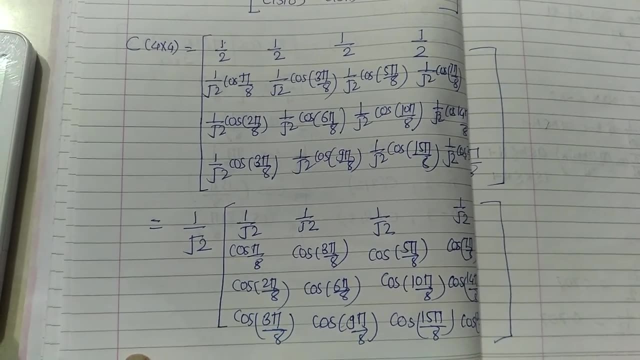 on the transform- sorry, on the image- to convert the image from one form to the another form. So thank you for watching my video. Please subscribe, share and like my video, Thank you. thank you very much. 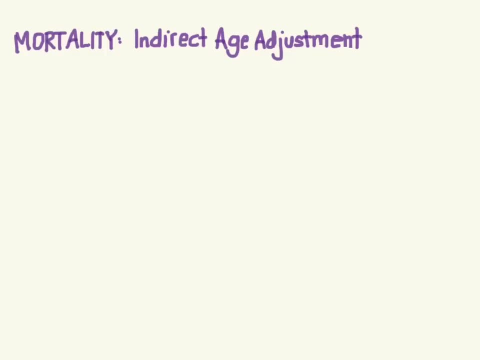 Now for the next video. we're going to talk about mortality and indirect age adjustments. Indirect age adjustments are good when you're missing some data, like you don't have the age-specific data for one of the two groups, And so we're going to do this indirect adjustment in order to account for that.